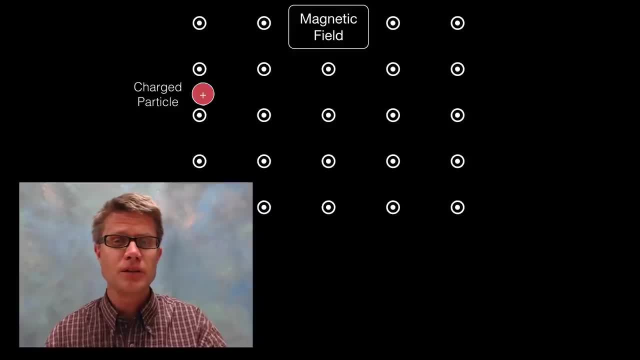 have a charged particle that has no velocity, It is just going to go away from us, It is just sitting there. Is there a magnetic force acting on that charged particle? The answer is no. If it is not moving there is no magnetic force. But as it moves it has a velocity vector. 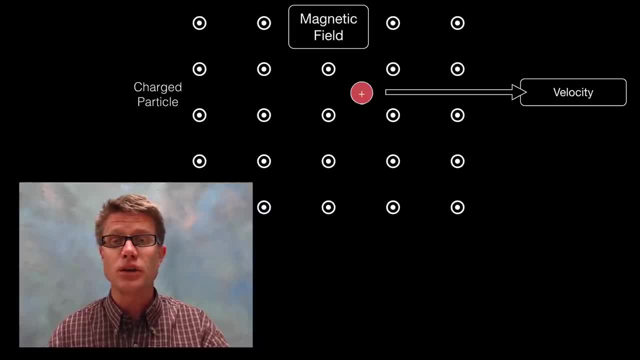 And if you are ever moving as a charged particle through a magnetic field, then you are going to have a force applied to you And we call that the magnetic force, or F sub n. Now, things that you need to remember is that it is a perpendicular line between the magnetic force. 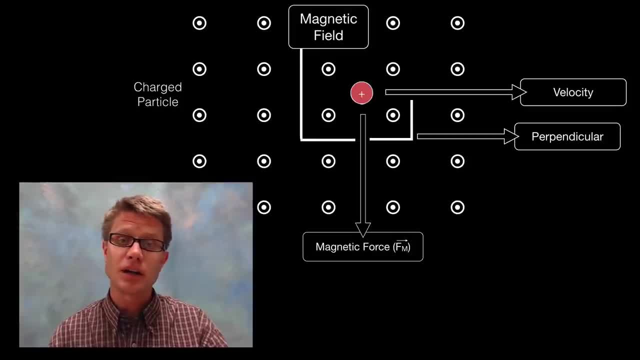 and the velocity. And it is also perpendicular between the magnetic force and the magnetic field. But the velocity vector and the magnetic field vector don't have to be perpendicular to each other. How do we calculate the magnetic force? Well, there are only three things: that 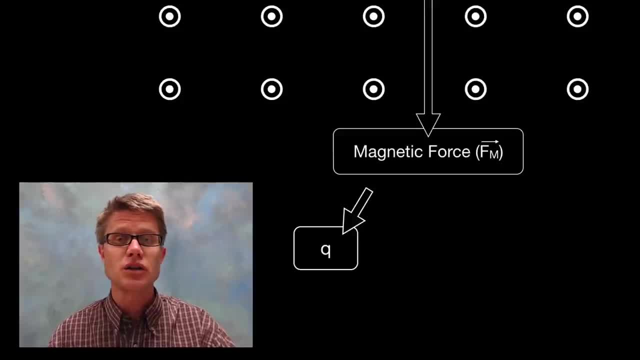 really deal with that. The first one is going to be q, That is going to be the charge of that particle. In this case it would just be the elementary charge. We then have the velocity vector, or the speed of the particle, And then we are going to cross product that. 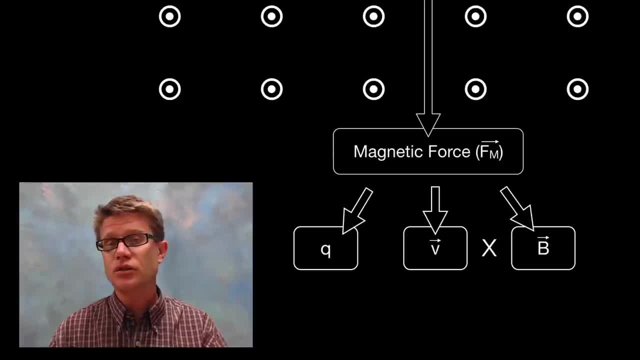 with the magnetic field. And what is a cross product? Well, these two vectors. when we multiply those together, we are going to have a force applied to it And we are going to get the going to get a third vector that's going to move in a different dimension. And I've got 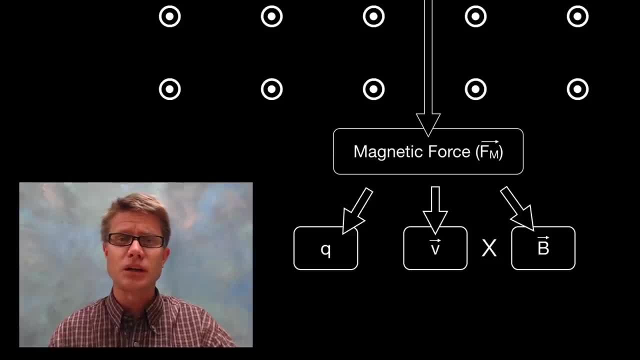 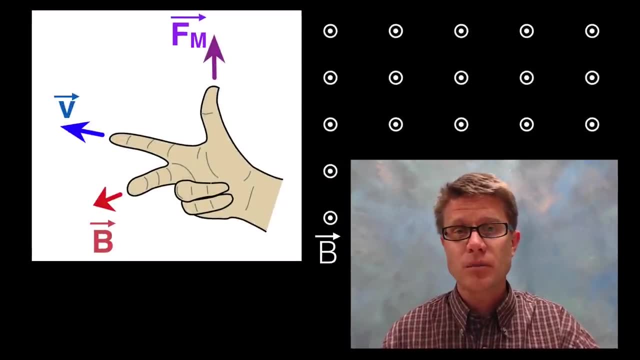 an animation that's going to show you that. Now, depending on that angle, we can get different amounts of this magnetic force. And so we use sine theta to figure out how much that's going to vary over time. And so let's say, we have a magnetic field like this: You can 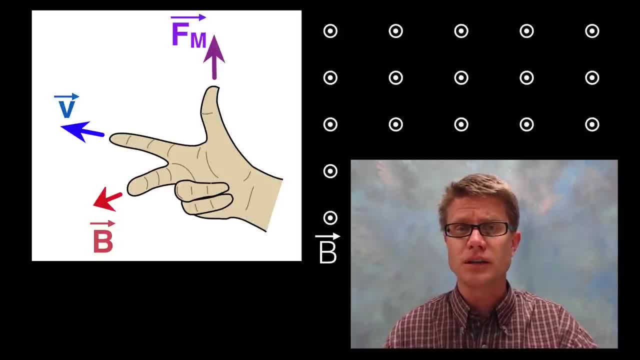 see that it's coming at us. To figure out where that magnetic force is acting, you have to use the right hand rule, And so it takes a second to get this figured out, But I'm going to hold my fingers out like this. So I've got my index finger pointed out, That's. 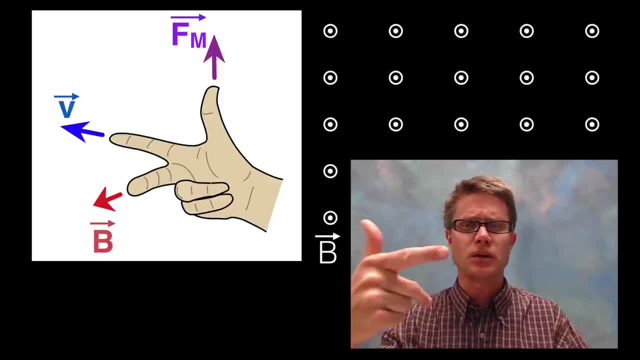 going to be the vector of the velocity. So, in other words, where that charged particle is moving, I then have my middle finger moving at 90 degrees to that And that's going to be the magnetic field, And then the force is going to be your thumb, And so you try. 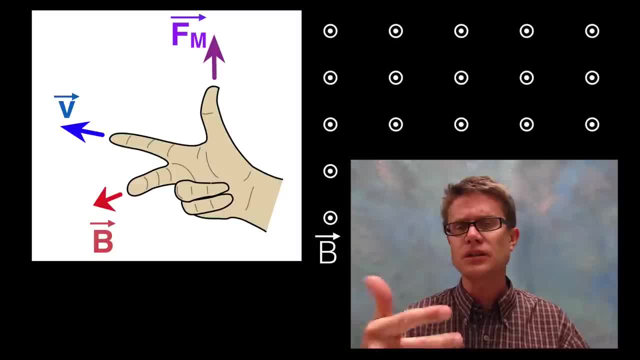 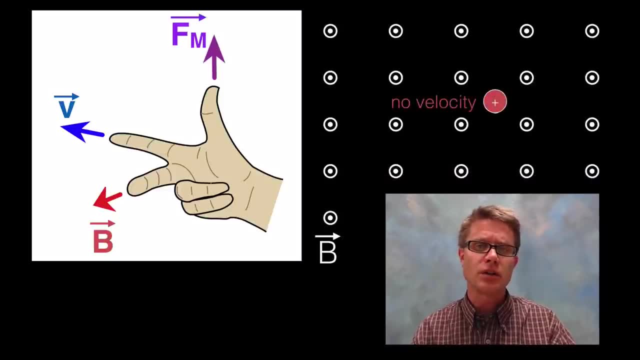 to make these three dimensions with your finger And you can solve really intense problems like this. You might look like an idiot as you're doing that, but it's worth it. So let's say we have a charged particle that has no velocity and it's in this magnetic field. 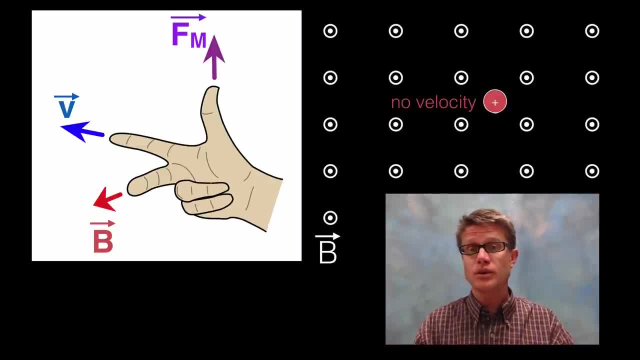 How big is our force going to be? This is going to be the vector of the velocity, So to be. Well, we are not going to have a force. Again, if it is not moving, there is no force. And so let me give you a harder problem. Let's say we have a magnetic field like this and 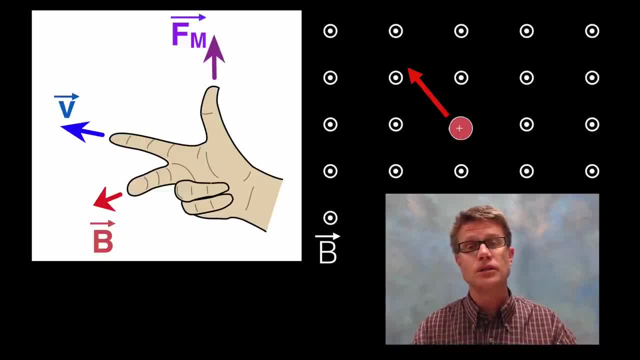 we have a charged particle, a positive particle that is moving up and to the left, And so how do you figure out where that magnetic force is going to be? Well, first of all, make your hand like this, And then you are going to point your index finger in the direction. 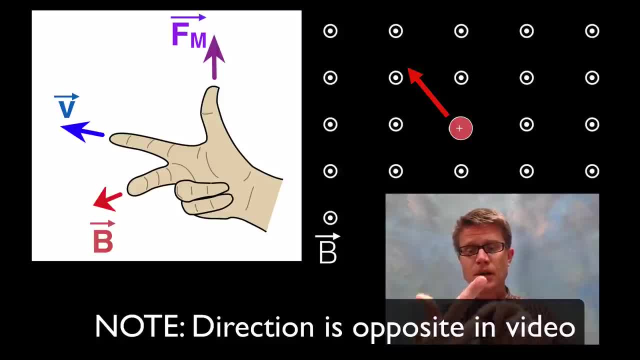 of that moving charge. So I am moving it up and to the left. Then you want to make sure that your middle finger, that magnetic field, is pointed towards you, Because you can see on this diagram that the field is coming towards us. And so once I have got that in order, my 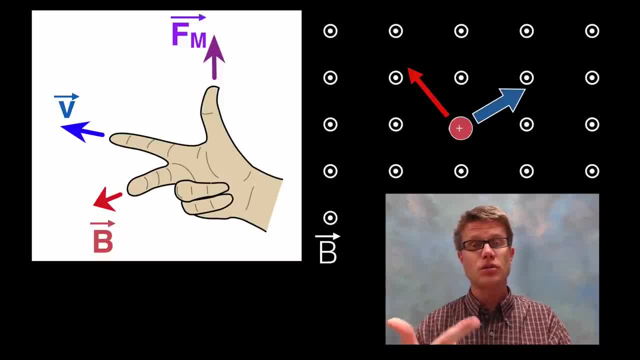 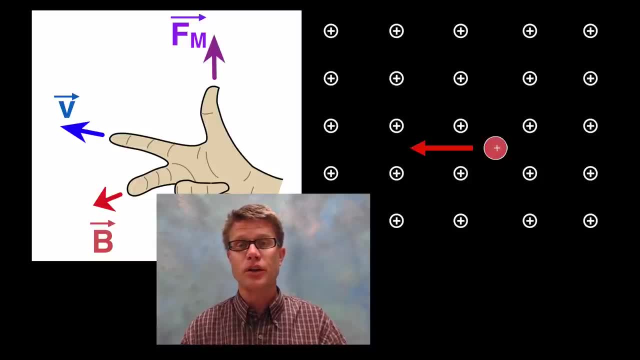 thumb is going to show me the magnetic force And so that is going to go up and to the right. So that was pretty easy to solve. Let's go to another one. Now we have got a different magnetic field And let's say that that charged particle, that proton, is moving from right. 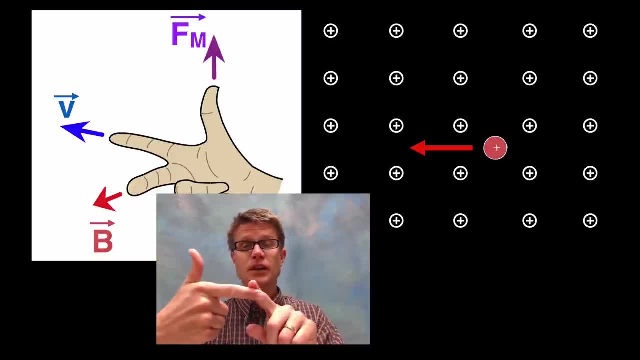 to left. How do you solve this? one Again, stick your finger towards the left. That is the movement of the particle. Now the magnetic field is going to move up and to the left. Now the magnetic field is not coming towards you, It is going away from you. So I have to turn my hand like this: 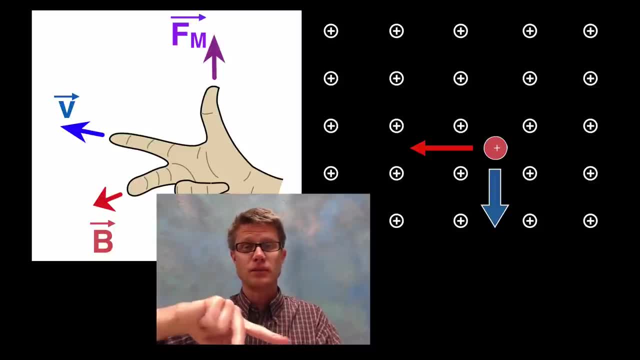 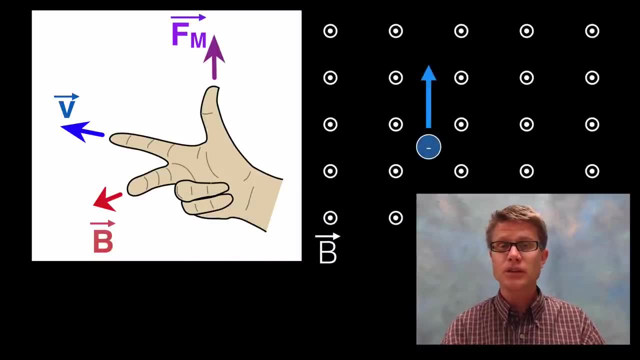 And now, where is the magnetic force? Well, you can see that that is going to be acting down. What if we have one like this? So we have got a different magnetic field. What if we have an electron moving? Okay, So if you have an electron moving, there is two ways. 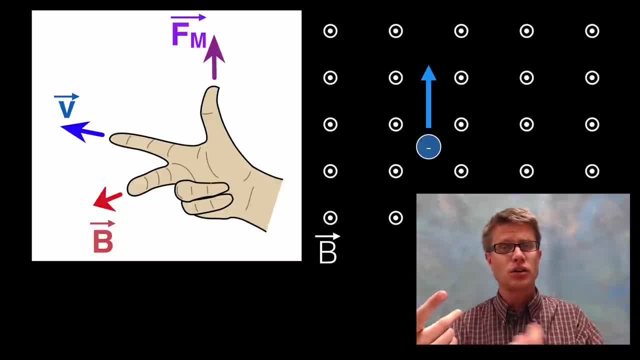 you can go at this Number one. you could just use your right hand and then just turn the force around when you are done, Or you have got a left hand And the left hand is going to work great. So I am going to point my index finger in the direction of the movement. 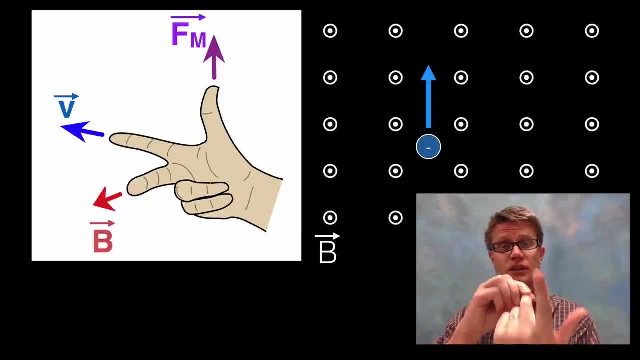 of the electron, Number two, the magnetic field. my middle finger, in this case, is going to come at me, And so where is the force? Now, the force is going to be to the left, And so if you know the magnetic field and you know the direction, you can always figure out where that magnetic 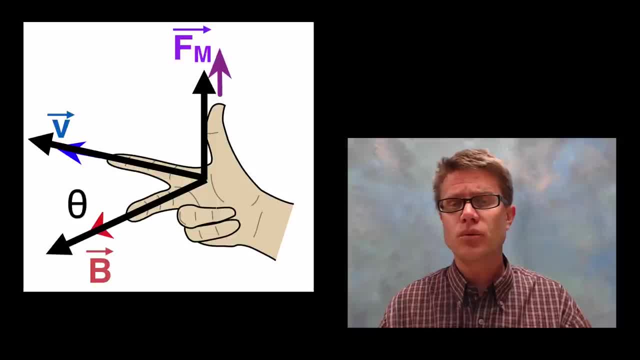 force is going to be. Now, the angle, as I said, is between the velocity and the magnetic field is not always 90 degrees, And so we call that theta, And depending on what that is, we are going to get a different amount of that magnetic force, And so those two are perpendicular. 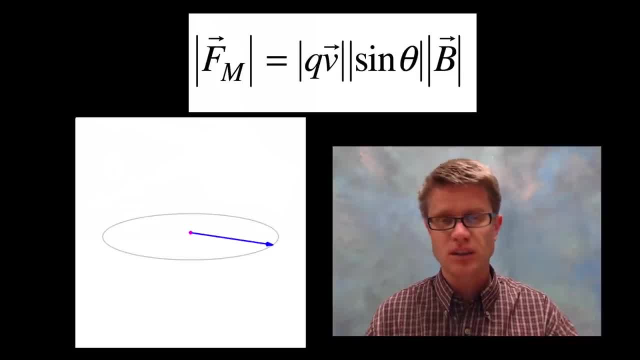 But the third one is not going to be perpendicular, And so here is our equation. It is a little scary, but it is not that bad. Q is going to be the charge, V is going to be the velocity, And then this is a cross product between the two, And so let's watch the animation before. 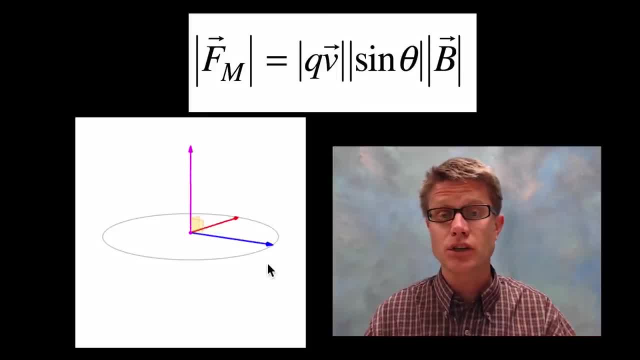 we get to the sine of theta. And so if they are pointed in the same direction- velocity and magnetic field- we have no force, But watch what happens. when they become perpendicular We have a greater force, or magnetic force If it moves to 180 degrees. what is our magnetic? force. at this point It is going to be 0. As I move it back, it is going to be 0. And then we have the force. So we have a greater force. So we have a greater force If it moves. 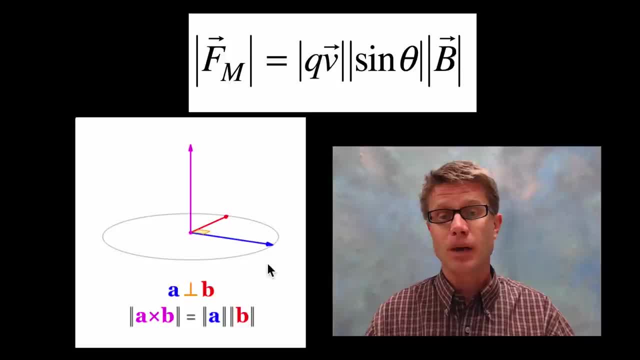 to 180 degrees. what is our magnetic force at this point? It is going to be 0.. As I move it back to 90 degrees, then it is going to be at its maximum at this time, And so by using this sine theta in the middle, we can figure out how much this cross product in other. 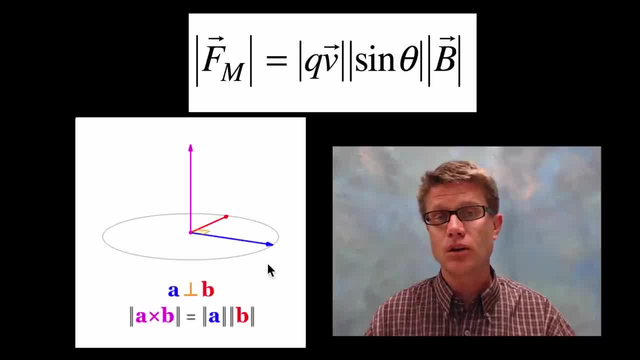 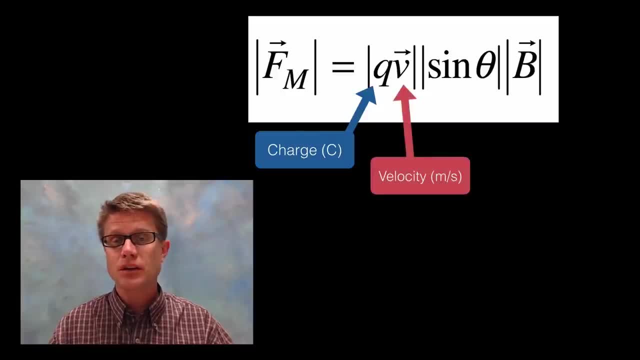 words, multiplying the velocity times the magnetic field is affecting the overall magnetic force, And so the parts of this formula are: Q, which is charge measured in coulombs, V is going to be the vector velocity, That is going to be in meters per second. And then we have 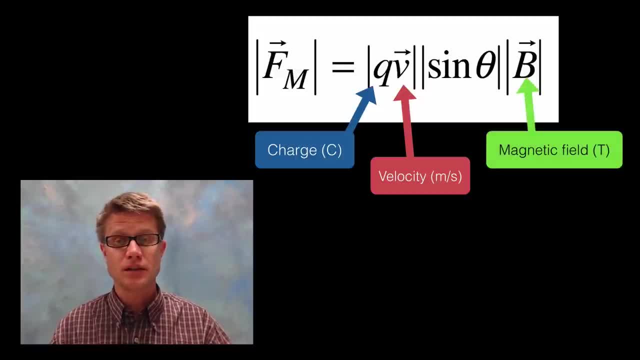 B, which is going to be our magnetic field, And we measure that in teslas, And then as we solve for the magnetic force that is going to be measured in coulombs, And then as we solve for the magnetic force that is going to be measured in teslas, And then as we solve, 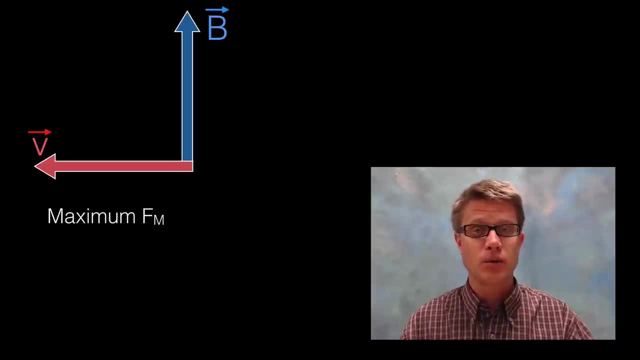 for the magnetic force that is going to be measured in newtons. And so let's get to that theta and the sine of theta. Where is that coming from? Well, let's say that our magnetic field and our velocity are perpendicular to each other. We know that that is going. 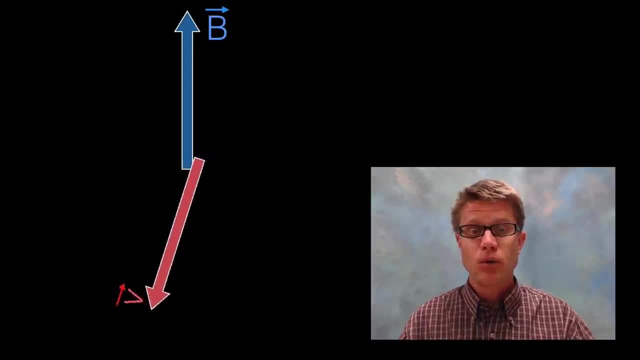 to be the maximum amount of magnetic force that we can get. What if it is this direction? They are in opposite directions. Do you remember what our magnetic force is going to be here? It is 0. And if they are both moving in the same direction, it is also going to be at 0.. 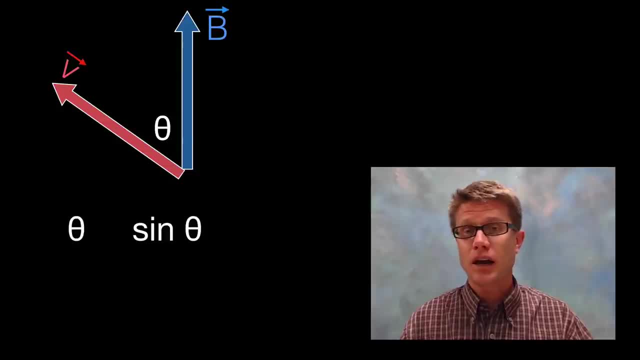 And so if we just choose that angle to be theta and then we have sine of theta, look what numbers we are going to get. So if it is a 0 degree angle, sine of 0 is going to be 0. There is going to be no magnetic force. Likewise, sine of 180 is going to be 0. But 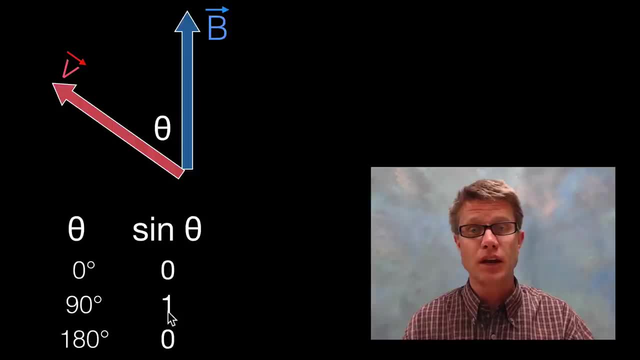 if we are at 90 degrees, that is going to be 1.. And the AP folks say that you should really understand 0,, 90 degrees and 180.. But the sine makes sense to me and it should make sense to you as well. What does our angle look like right here? Well, that is around. 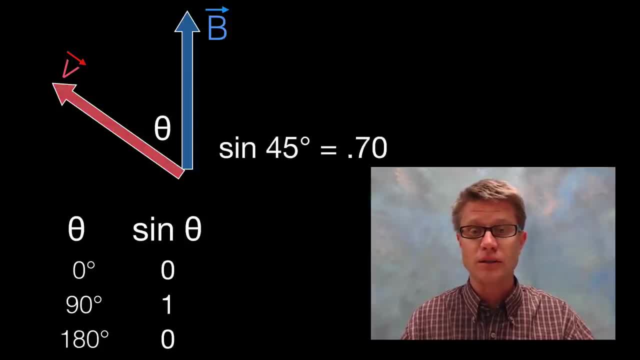 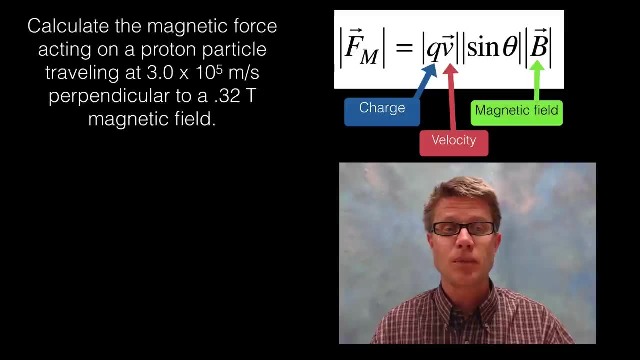 a 45 degree angle. So what is the sine of 45? It is just going to be 0.70.. It is going to be somewhere between 1 and 0.. And so if we do a problem like this, calculate the magnetic force acting on a proton traveling.